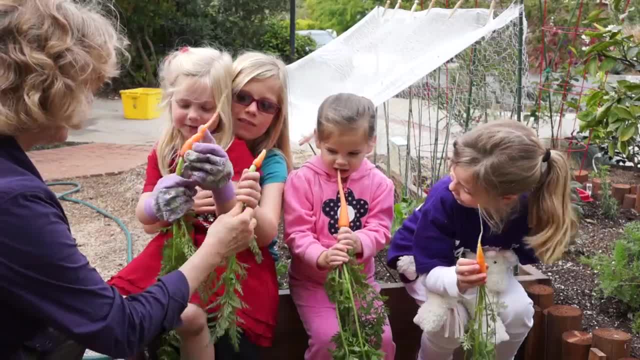 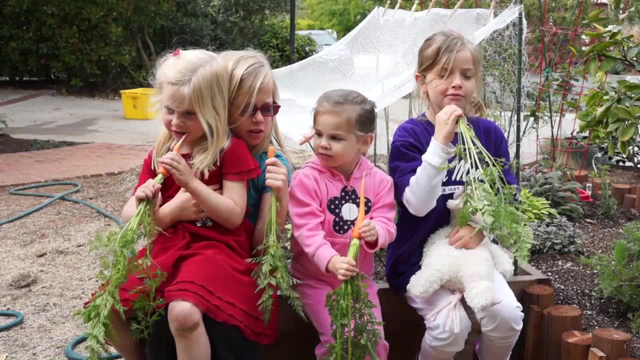 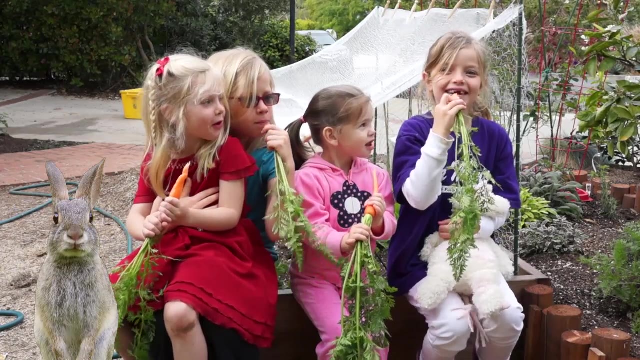 I want this one. I like this one. I'll have the little one. Tell me what you think. Yum, Yum, This is good. Yum, I'm a bunny rabbit. Good job, Same, And maybe we should make some more. 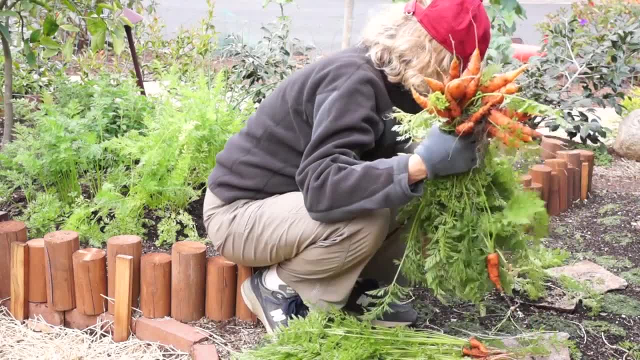 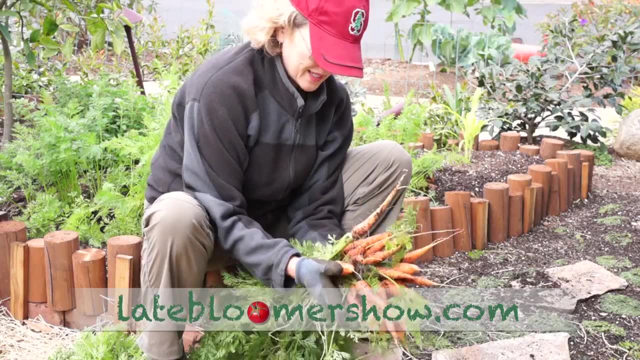 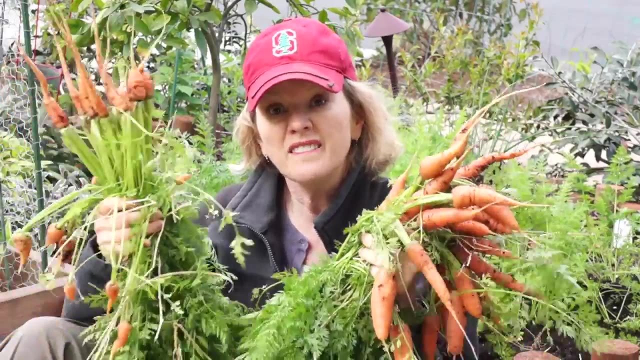 The neighbor girl's endorsement told me it was time to harvest. Here's my first batch. Look at that, It's a pretty good crop. We're going to have carrots tonight. This illustrates the importance of thinning out your carrots. All these guys. they don't develop. 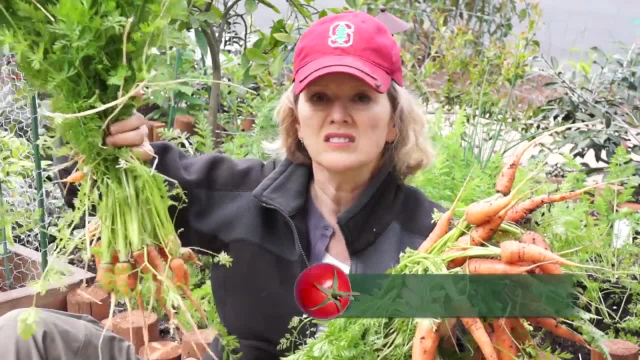 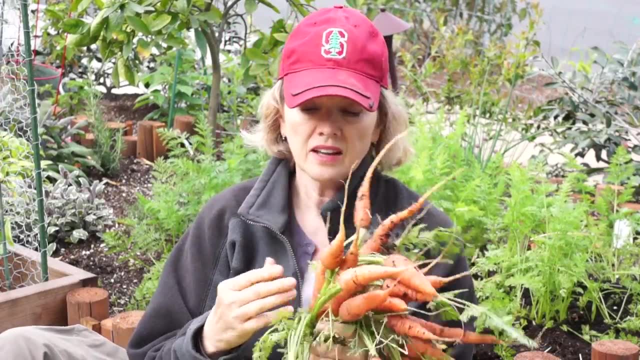 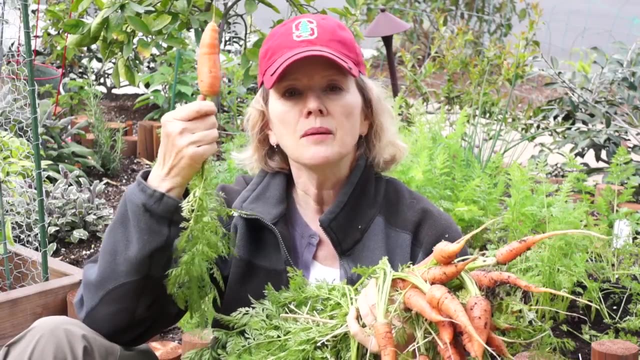 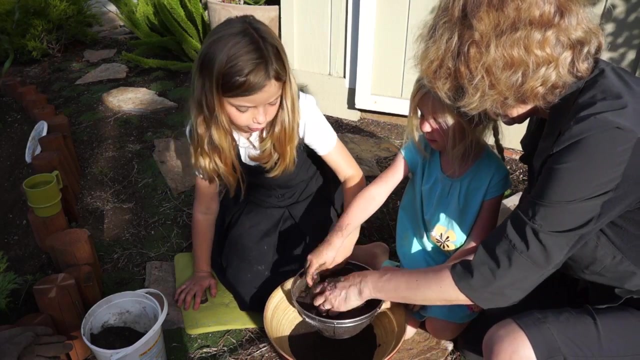 All the energy goes up into these massive stalks, They're not really edible. So by thinning, you give your carrots a great chance to develop under the ground. Look at that one: It's like a perfect carrot. The girls love to garden, so we planted more carrot seed. 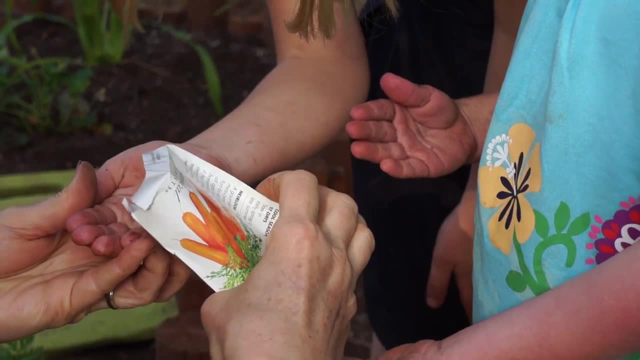 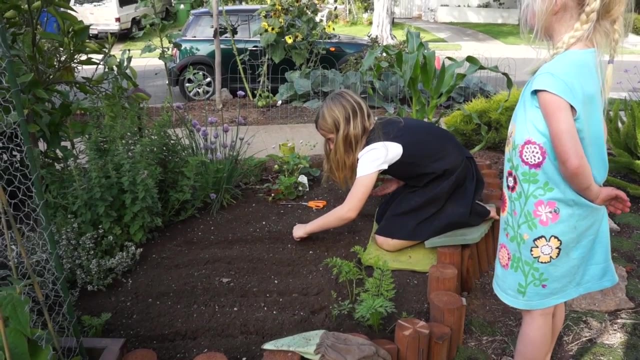 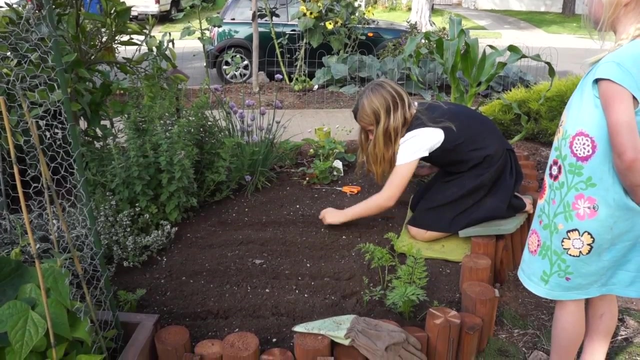 First we sifted the compost Tiny seeds into tiny hands- That's how many you put in that entire row. Courtney was doing a careful job of planting and Ashley was waiting her turn. Then their dad called them in for dinner. Sure, 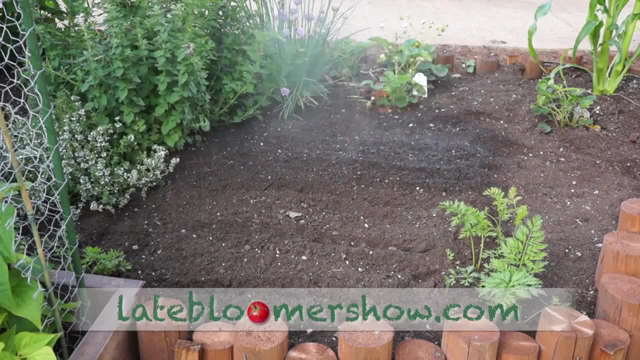 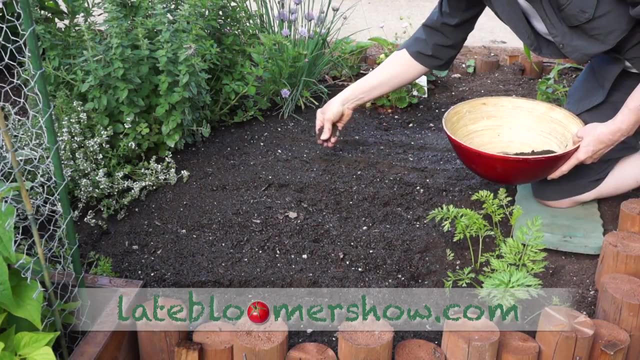 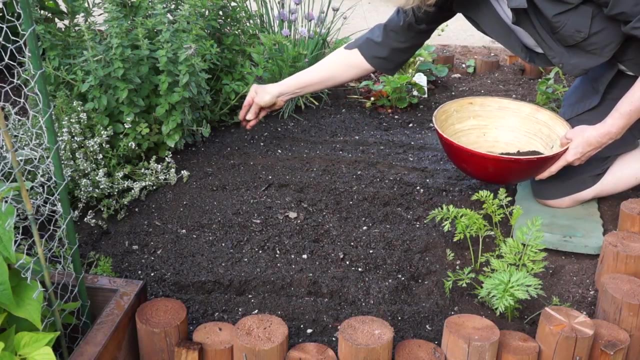 I finished the job. It would have been smarter to wet the dirt first, but You just put a quarter of an inch, So I have sifted my compost. It's very fine, And I can get a nice even quarter of an inch on top. 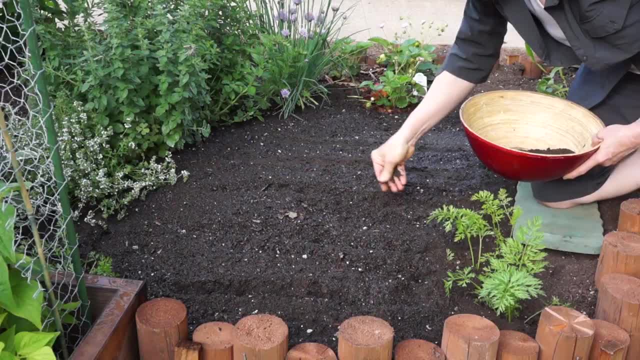 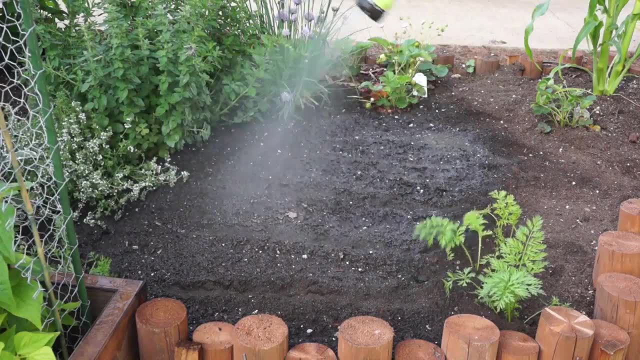 You don't want these tiny little seeds to be too buried, otherwise they won't sprout. And a final misting All done Just when my neighbors strolled by. Hey ladies, Hello, How you doing today. Very good. 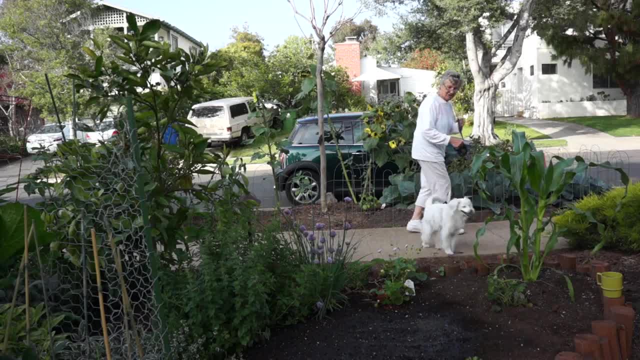 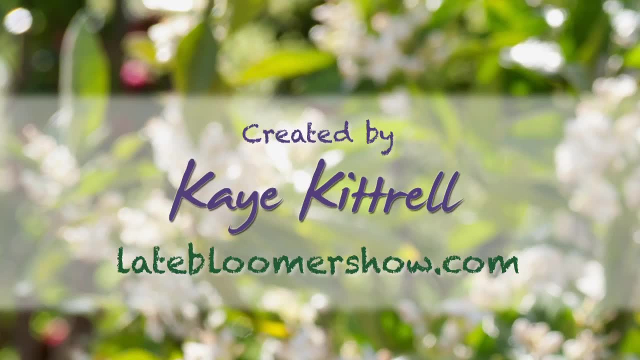 What a nice garden you have here. Oh, thank you Vegetable, and I'm Kay and I'm a late bloomer. I want a carrot. I want a carrot, Me too. You had a carrot, No, but I want another one.